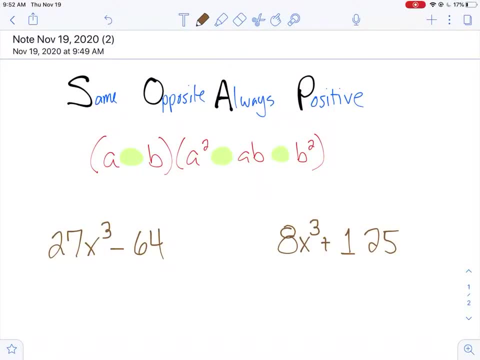 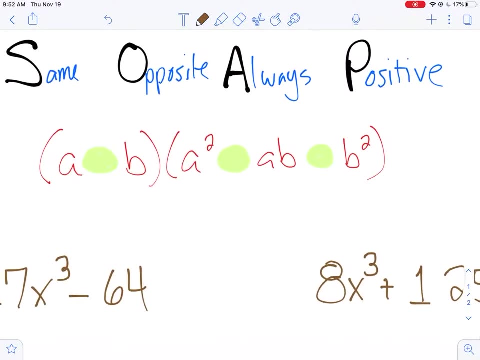 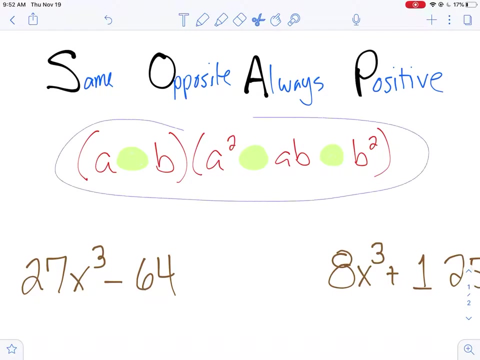 I'm going to go over sum and difference of cubes today. Now I'm going to be using this acronym: same opposite, always positive. You will notice that when you factor out a sum or difference of cubes, it's always going to take the form I have here: A blank, B in parentheses, then A squared, blank, AB blank, B, squared. So I'm going to be using this a few times today in the course of these two problems. 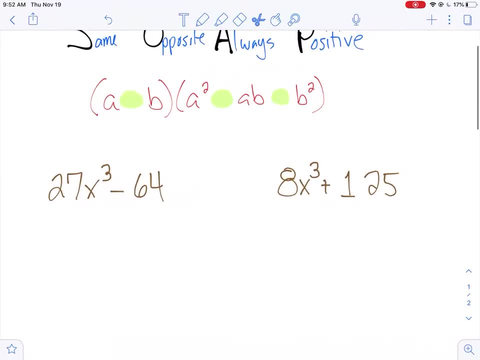 So you'll notice, here I have 27x to the third and 64. Now my first step is: I want to find the cube root of both of these. Cube root of 27x to the third is going to give me 3x, That's going to be A. Next, I want to find the cube root of 64. That's going to be 4, which will be B, And now all I have to do is basically fill in the blanks. 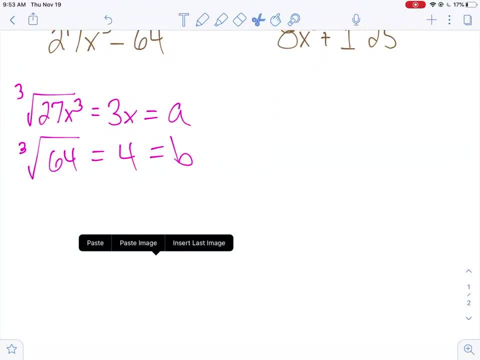 So I'm going to take my formula and pop it down here. So for A, I have 3x, For B, I have 4.. Now this would be 3x squared. Bear in mind, Make sure you're squaring that whole thing. I would have A times B, which would be 3x times 4.. Then I have B squared, which is 4 squared. Now where are my operations? This is where it comes in. 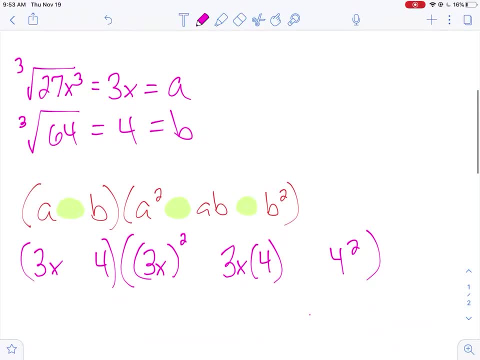 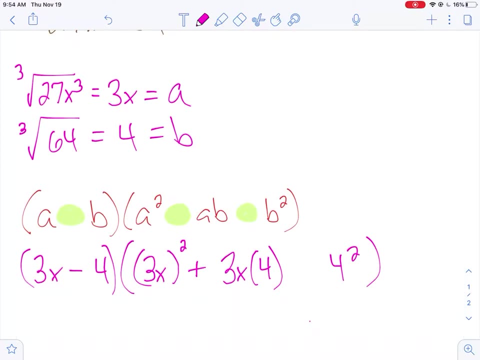 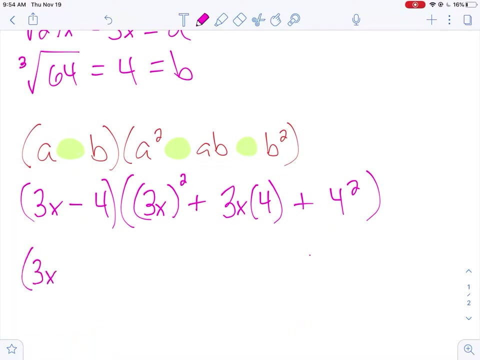 Same. So, since this is a subtraction problem, I'm going to use subtraction Opposite. Opposite of subtraction is addition. And then the last one, always positive plus. So I'm just about done factoring it. All I have to do is simplify it: 3x minus 4.. 3x squared Now, remember you're going to square the 3 and the x, which will give you 9x squared. Then 3x times 4 gives me 12x. 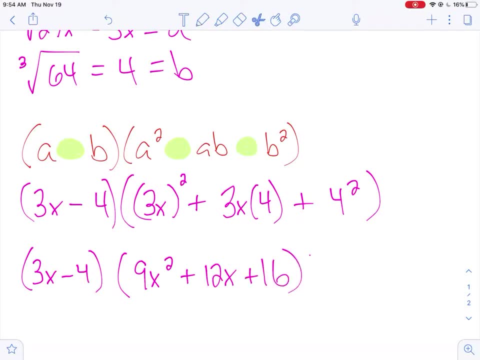 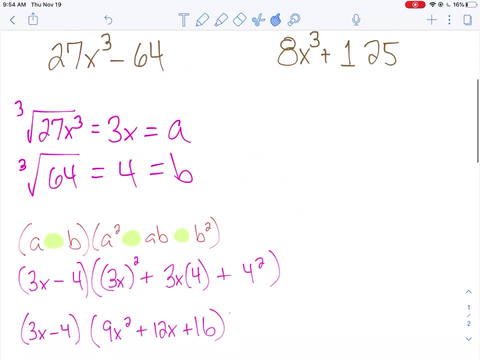 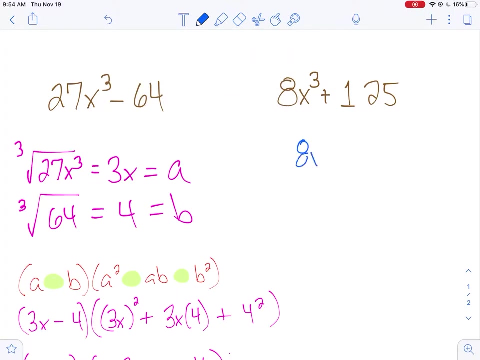 4 squared gives me 16.. You know it's not that bad. Don't be intimidated by this. It's relatively easy once you get the idea of the form and the formula. So let's do the next one. This one's going to be a sum: I get 8x to the third. Find the cube root of that, which would be 2x. That's going to be A.